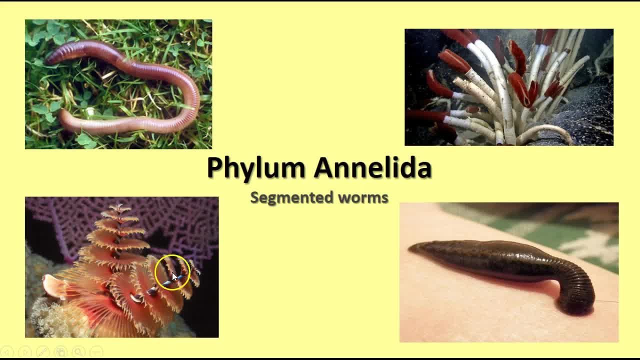 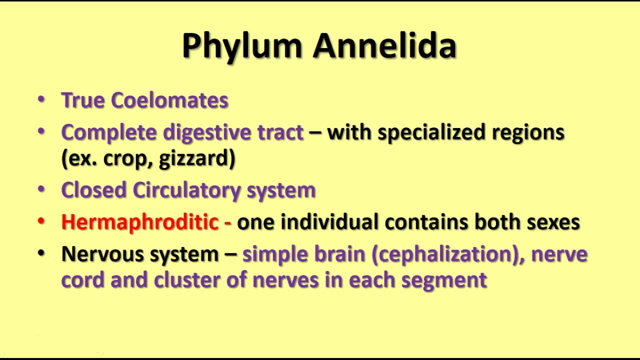 ocean and this is a fan worm that is also a marine organism. So there are lots of different members of this phylum. as we'll see, Phylum anelida are true coelomates. They have a true coelom, that is. 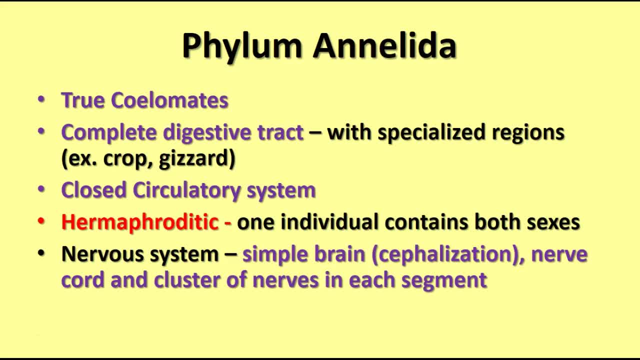 between layers of mesoderm. It's completely surrounded with mesoderm tissue. They have a complete digestive tract with specialized regions like the crop and the gizzard. A crop is a part of the digestive system that stores food while it's waiting to pass through the gizzard, which is a 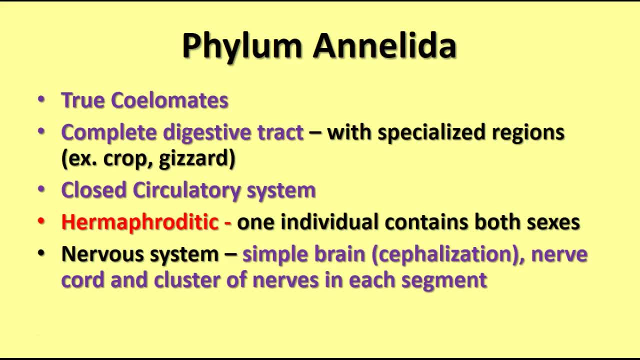 grinding organ that can grind up hard pieces. Since analids often eat dirt, then having the ability to grind up pieces that might be hard is definitely a good advancement for them. They have a closed circulatory system. This is similar in some ways to your circulatory system, in which the blood remains in vessels all. 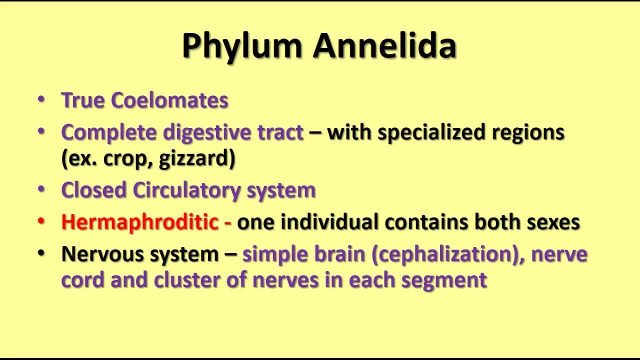 the time and doesn't come in contact, direct contact with tissues. The analids are hermaphroditic, That means one individual contains both sexes, and this is an advantage, as we talked about before, for organisms, the animals that are relatively solitary, so that anytime they happen to come, 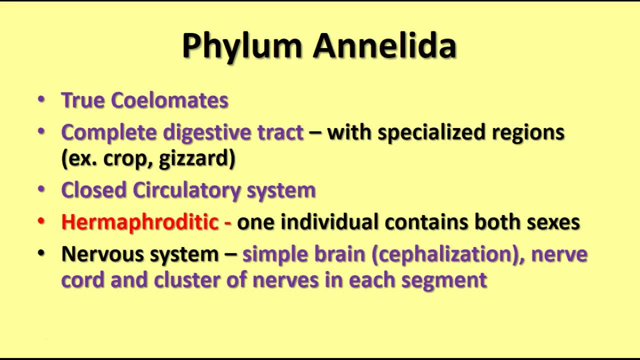 across a member of their species, they should be able to exchange gametes, even though they don't often run across another member of their species. In terms of a nervous system, they have a simple brain. In other words, there is cephalization, or the development of a head region in analids. 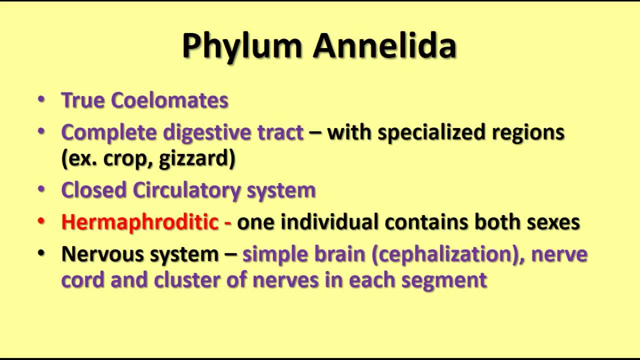 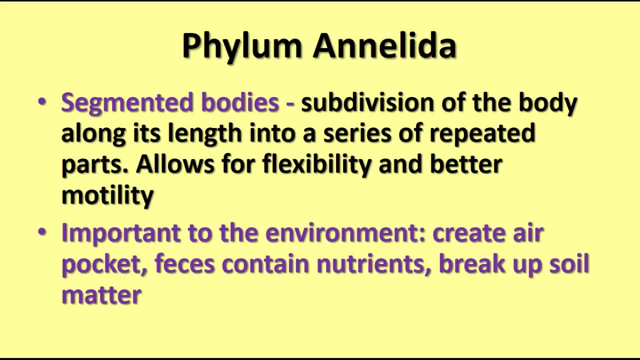 and they have a nerve cord and cluster. There is a structure of nerves in each segment of the body. Another advancement that analids have that hasn't been seen in any of the previously discussed phyla is that they have a segmented body. Their body is subdivided along its length into a series of repeated parts. For the analid, this 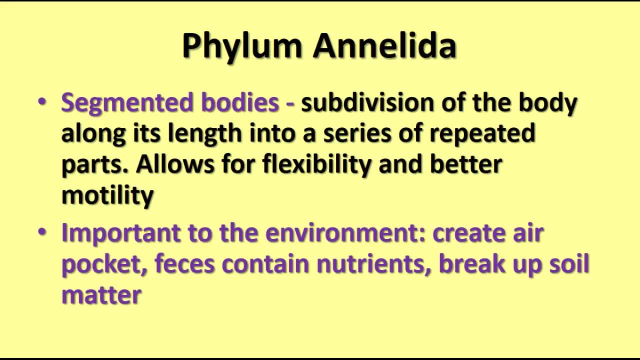 allows for flexibility and a better motility, because each segment can move independently as long as it's connected to the others. The analids are important to the environment for a number of different reasons. They create air pockets in the soil, their feces contain nutrients and they can help break up soil matter. so earthworms in 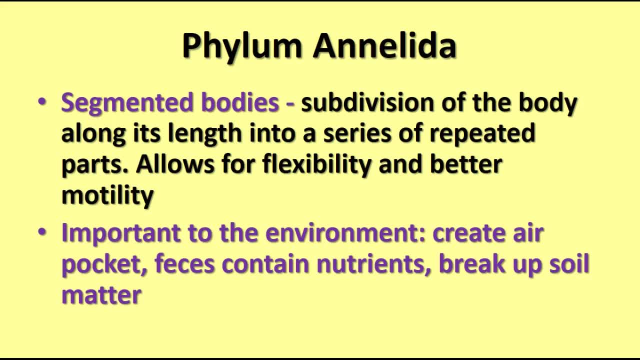 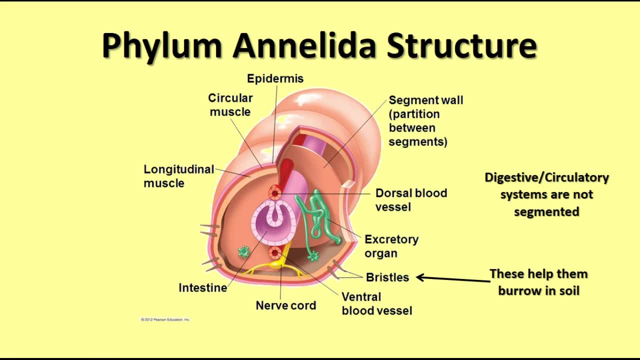 particular or other analids that live in the earth are very important to maintaining the environment and making conditions better for plants that grow in the soil. Here we have a cross-section of an analid showing some of the internal structure. here Notice that we cross walls or segment walls, that are partitions in between segments. 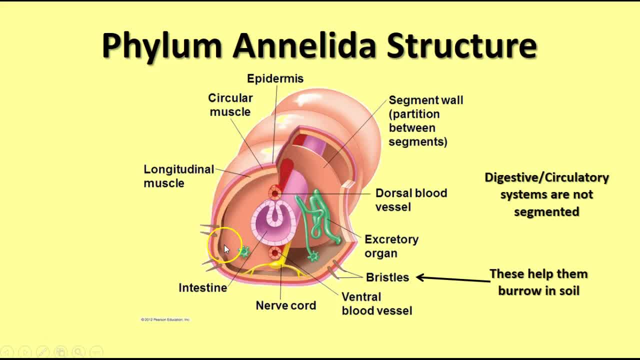 There are circular muscles that go around this way and there are longitudinal muscles that go lengthwise And if you've ever seen an antelope crawl, an earthworm crawl, you can see that the contractions of both of those muscles together helps it move forward. 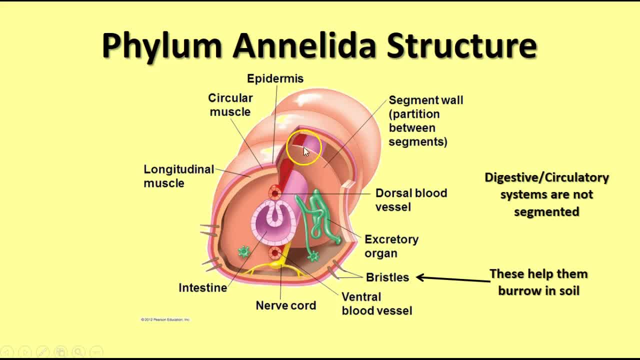 There's a dorsal blood vessel and a ventral blood vessel that travel from the aortic arches in the anterior part to the rest of the animal. The digestive tube, or the intestine, travels through the entire animal. There are excretory organs in each. 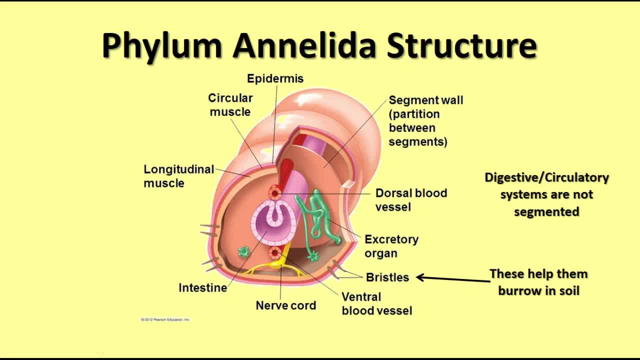 segment that are called nephritia, that help filter out a nitrogen-containing waste from the blood and tissues of the animal. There's a ventral nerve cord that is connected to the ganglia in the front or the anterior end of the animal And finally, there are bristles that you often find. 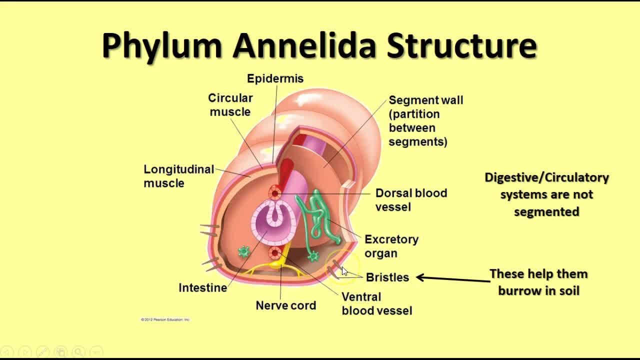 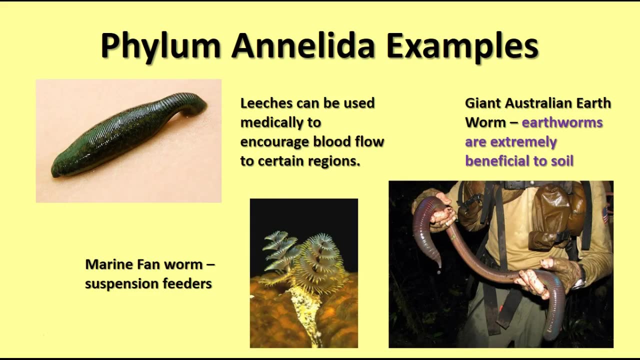 on the bottom edges, like this on the ventral edges, that actually help with burrowing down into the soil and gripping onto surfaces as they move from place to place. Some examples of aloe include leeches, which can be used medically actually to encourage blood flow in certain regions If 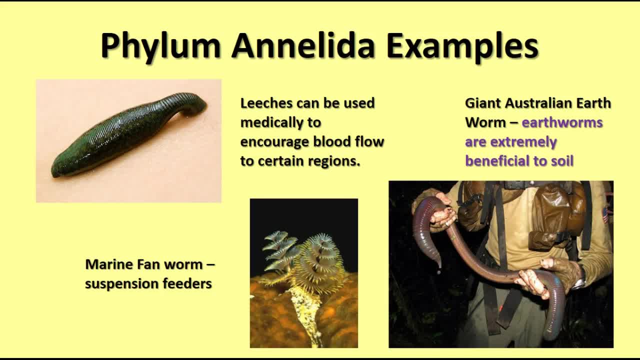 you have a portion of the body that has been limited in blood flow, either through a blood clot or through the reattachment of an amputated limb, like a finger or something like that. leeches can help actually promote blood flow into that area to keep it healthy. 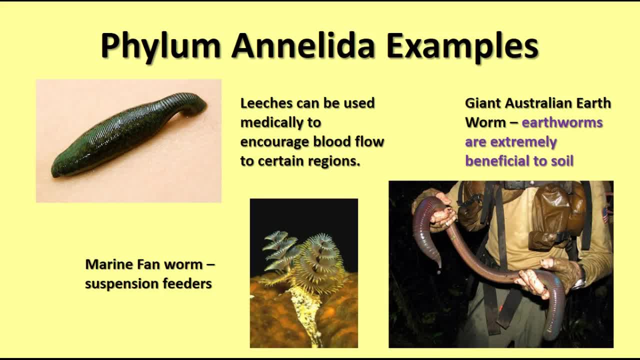 Marine fanworms are suspension or filter feeders, And over here on the lower right we have a giant Australian earthworm Now. earthworms are extremely beneficial to the soil. I'm assuming that these Australian earthworms that are so gigantic have the same effects, but it seems to me they're pretty darn big. 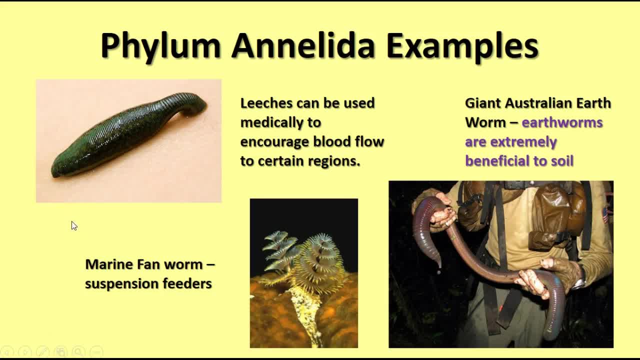 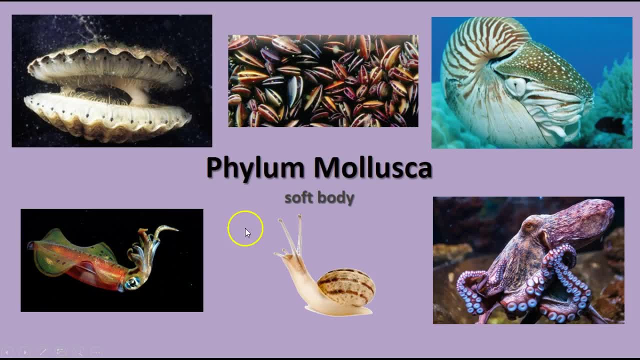 so I'm not sure what the difference is, But they do. they probably break up the soil deeper down than we have here in the US with our earthworms. The next phylum we'll discuss is phylum mollusca. The molluscs have soft 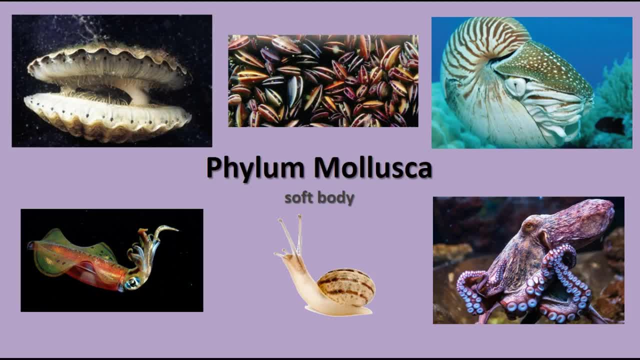 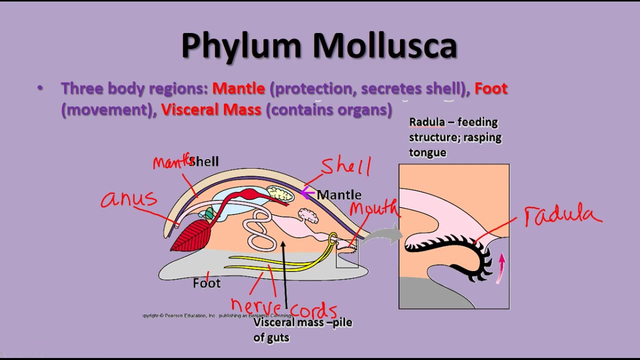 bodies, and most of them have a shell or two, And so this includes things like clams and squid and snails, octopi and another type of cephalopod like an octopoda. The molluscs have three main body regions: the mantle, the foot and the visceral mass. 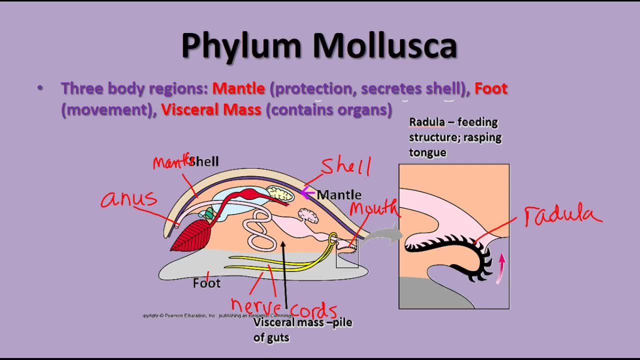 The mantle provides protection and secretes the shell. It's found, it's a layer that's shown in the diagram here in purple, that is just underneath the shell, and it secretes the shell on the outside. The mantle is also the part that secretes the mother-of-pearl, or the pearl, the nacre, that 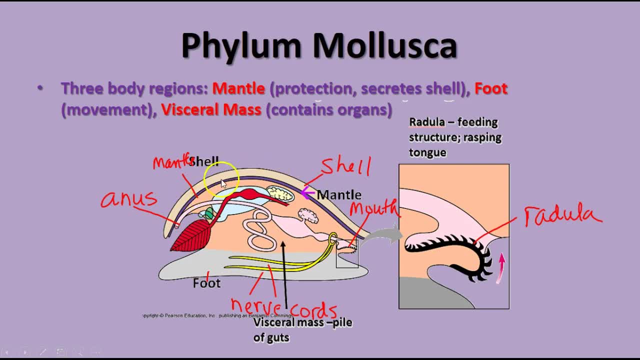 makes the pearl In clams when they get an irritant inside them. The foot is the organ that is used for movement. It could be a single foot, like we have here in this snail-like mollusk, or it can be divided into parts, like the arms or tentacles of a squid or an octopus. 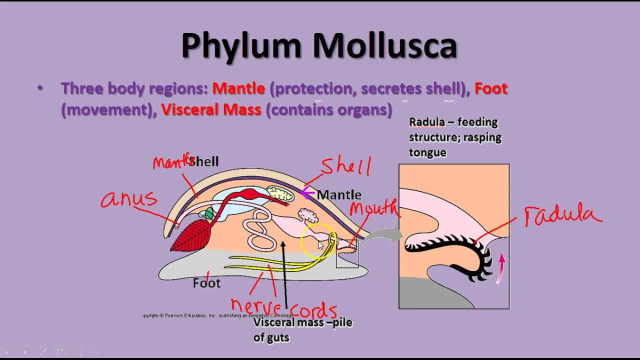 They have a complete digestive system inside their visceral mass, from mouth to anus. They have a respiratory system. They are open circulatory system. for the most part There are reproductive organs inside the visceral mass as well as in their cords And in the mouth region. they have some specialized structures in gastropods or snail, like animals. 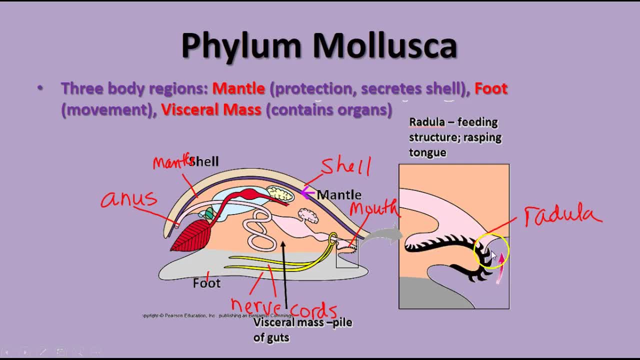 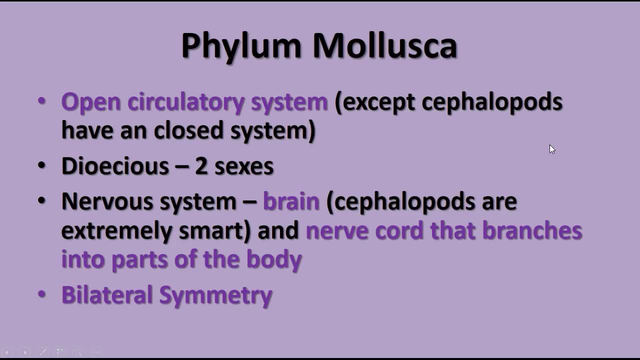 They have this rasping tongue like structure called arudula that helps actually break up food particles, like plants that they happen to eat. eat. Mollusks have an open circulatory system, except for the cephalopods, which we'll talk about in a minute. The open circulatory system means that the blood 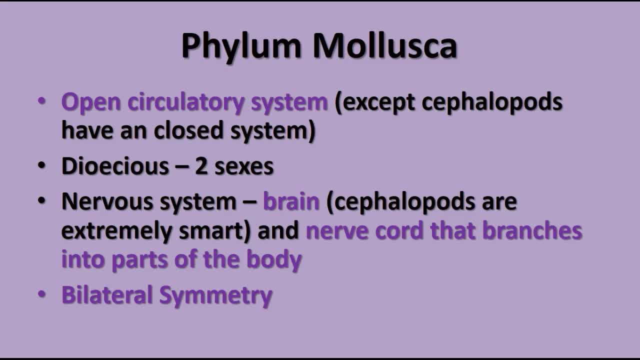 does not remain inside vessels all the time, but rather comes into direct contact with the body tissues for the nutrient and gas exchange that occurs between the blood and the tissues In your circulatory system, which is a closed circulatory system. the blood remains in vessels all the time and the 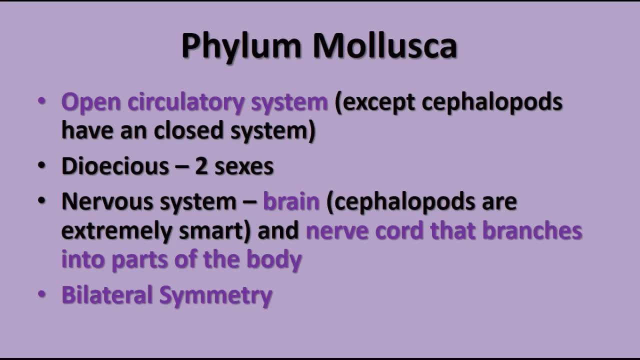 transfer of nutrients and gases and waste products occur via diffusion through the walls of the capillaries. The mollusks are dioecious, meaning they have two separate sexes: There are male mollusks and female ones. In terms of a nervous system, they have a brain. Cephalopods, especially, are extremely 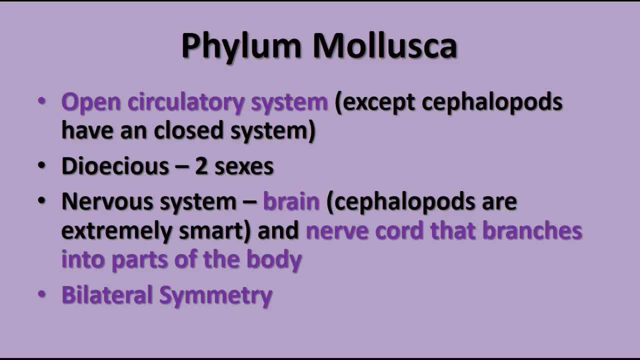 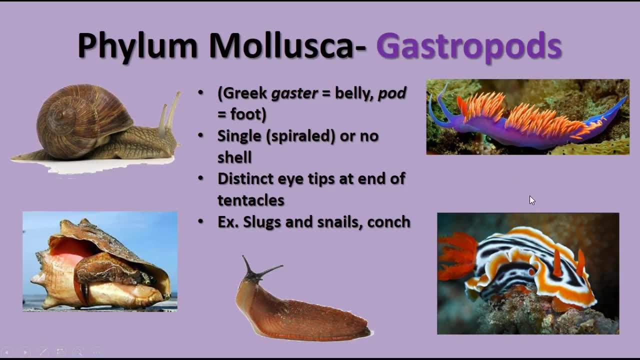 smart and they have a nerve cord that branches into the parts of the body. They also exhibit bilateral symmetry. There are three main groups of mollusks. First of all, the gastropods. Gastropod means belly foot or stomach foot. These are the single-shelled or no-shell. 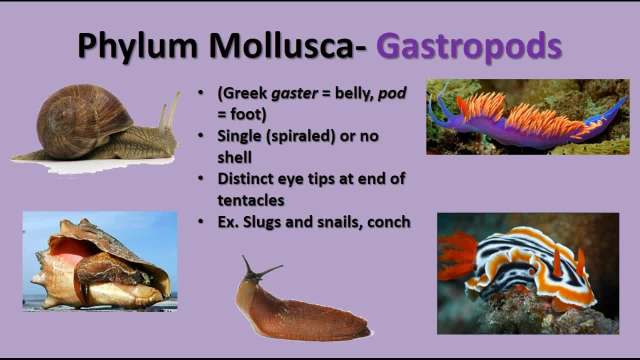 animals like snails and slugs. They have eye tips at the ends of their tentacles and this includes things like snugs, sails, snails, conch. These are some marine sea slugs that are in the same group. Conchs and other kinds of snails have. 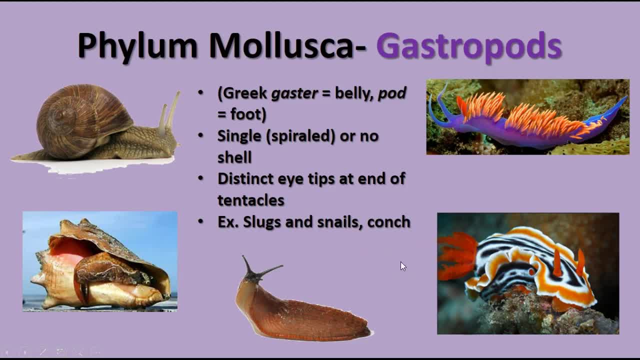 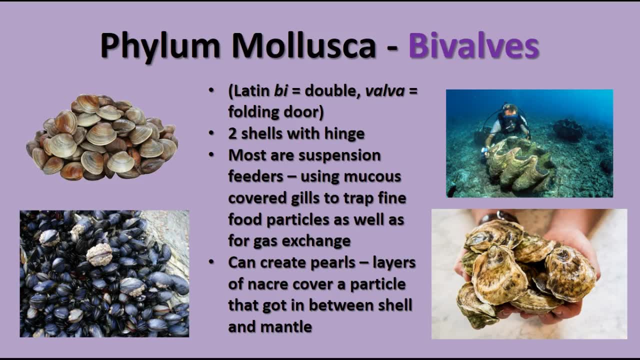 single shells. They are a member of the gastropods. The second group is the bivalves. Bivalves have two shells with a hinge that holds them together. Most bivalves are suspension feeders or filter feeders. They filter things out of the 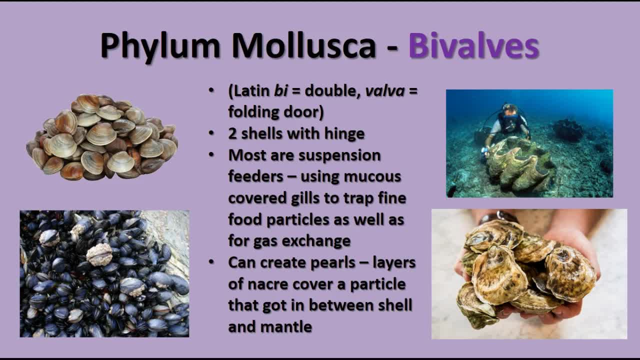 water with their mucus-covered gills, and the gills also take care of gas exchange. These are the animals that can create pearls. This is layers of the pearl material called nacre over a particle, an irritating particle like a piece of sand or something like that that got between the shell and the 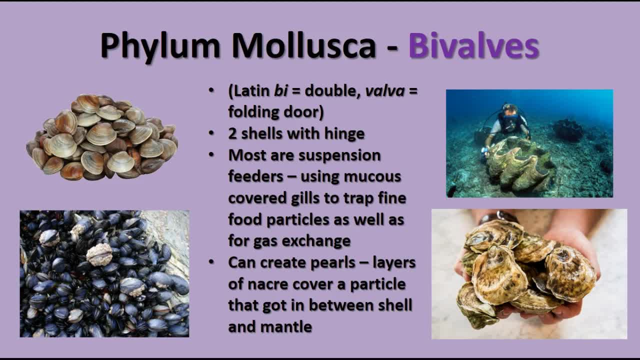 mantle. It's kind of like if you had a rock in your shoe. It gets very irritating when you walk on a little bit. Fortunately we have hands and we can take the rock out of our shoe, but oysters and clams don't have that. 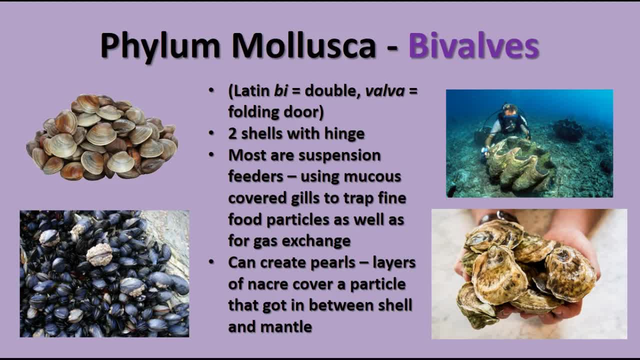 advantage: They don't have a hand that they can remove the irritant with, and so they can secrete the many layers of this really smooth substance called nacre that is like the pearl material Over this, over the irritant, so that it becomes less irritating to them. The 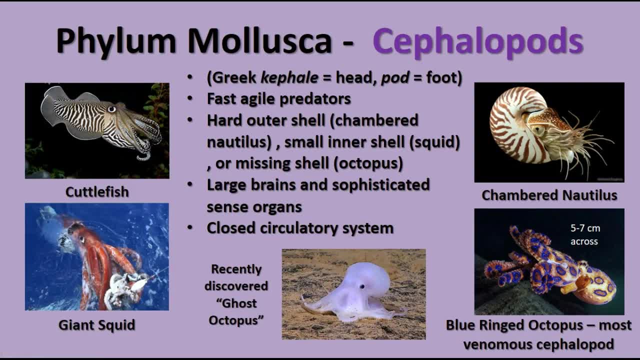 third group of mollusks is the cephalopods. Cephalopod means head, foot, and so their foot. the movement part of the body is actually divided into tentacles or arms and seems to be attached, or looks like it's attached to. 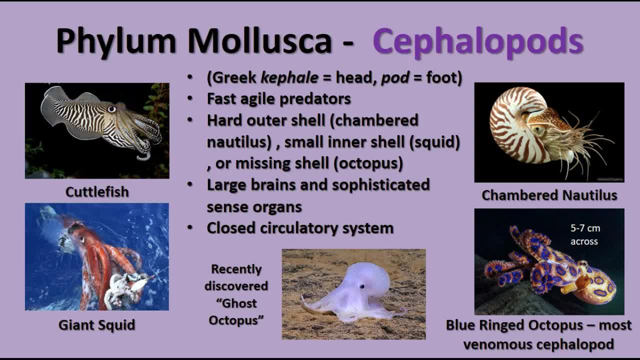 a head These have. these are very fast predators. They're carnivores, They're very agile, They can move really well. They can move to very narrow spaces. Those that have a shell include one species nowadays called the chambered nautilus, and it's a 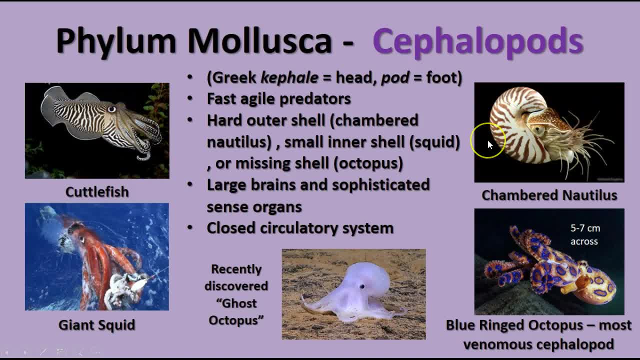 hard outer shell. They actually swim backwards by jet propulsion. They squids oftentimes have a small inner shell and the octopi don't generally have a shell. Octopi and cuttlefish have a small interior shell as well. They have large brains. 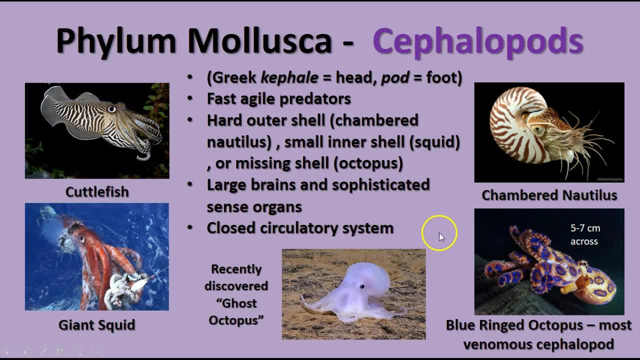 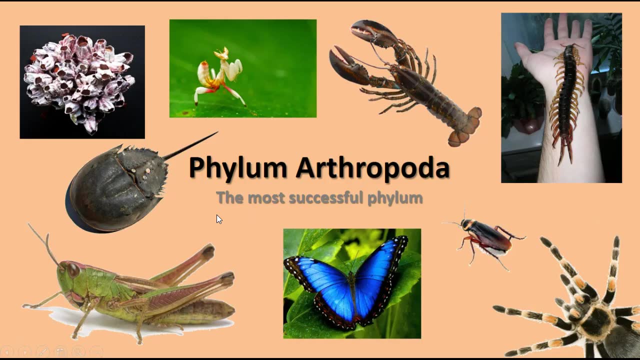 And very sophisticated sense organs. Their eyes work just about as well as yours and mine do, And they also have a closed circulatory system, which is a big advantage for an animal that is fast and agile like they are. The next group we'll discuss is the arthropods. The arthropods are the most 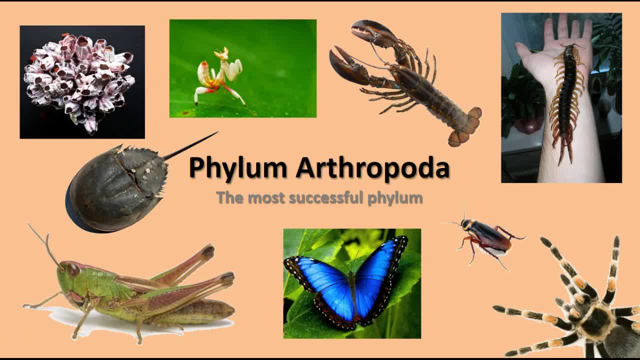 successful and the largest group of invertebrate animals. This includes many different things like insects, spiders, centipedes, horsey crabs and so forth, So we'll talk about the different groups of arthropods. Phylum arthropoda has. 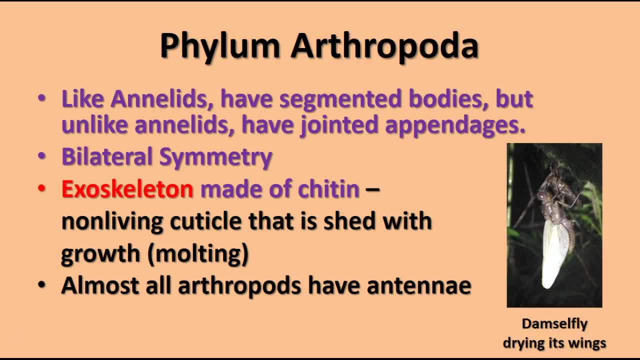 segmented bodies, like analids do, but unlike the analids they have appendages, arms and legs and antennas that are jointed, Meaning that parts of them can move independently of others. They have bilateral symmetry and an exoskeleton made of chitin. Remember the other time we talked about chitin was when we 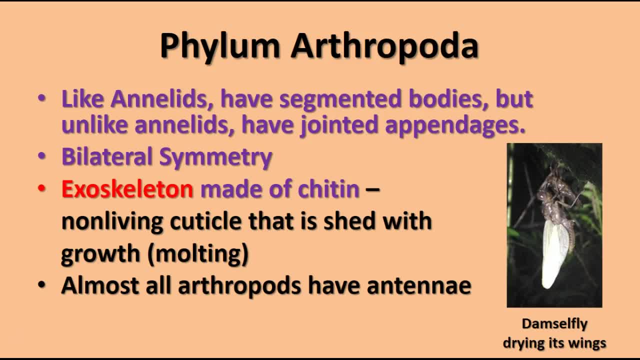 discussed fungi. The cut, the exoskeleton, is basically a non-living cuticle layer that is shed as the as the animals grow In order to grow, they actually have to shed their shell, first, their exoskeleton, then grow their soft bodies. 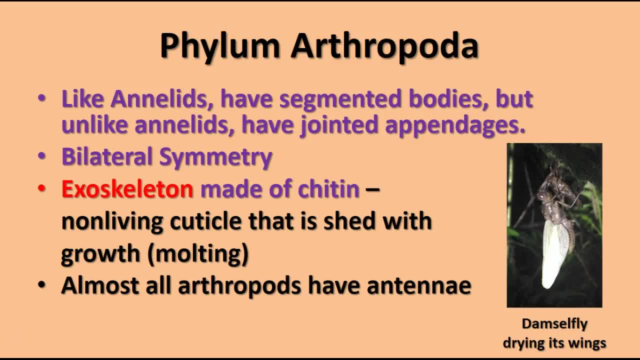 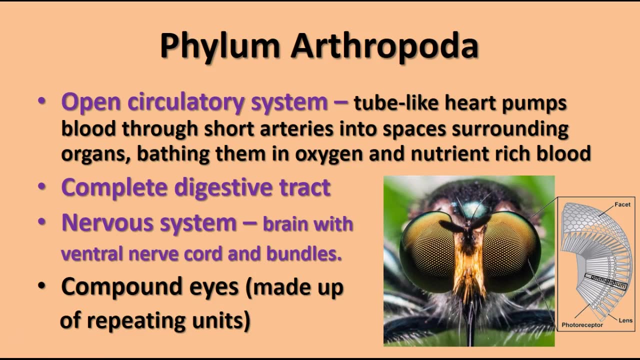 and then secrete a new exoskeleton. Almost all arthropods have antenna- either one pair or two pairs of antenna- and various numbers of legs and other parts. Arthropods have an open circulatory system like that that we saw in the mollusks. 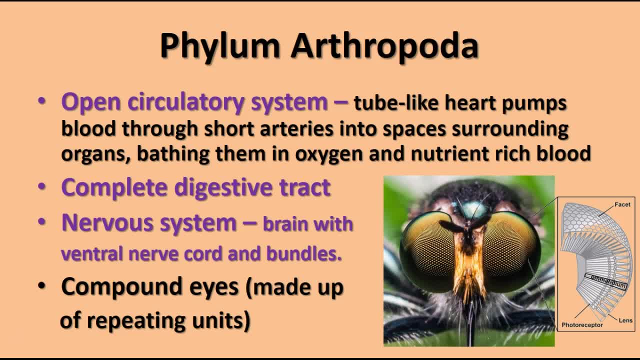 Their tube-like heart pumps the blood through these short arteries into spaces surrounding the organs- those are called sinuses- bathing them in oxygen and the nutrient-rich blood and then picking up waste materials. They have a complete digestive tract with esophagus, stomach and intestine and as well as the 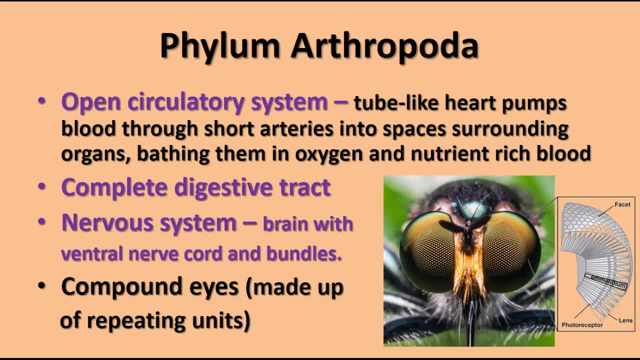 anus and other structures that may be present. They have a nervous system that includes a brain with a ventral nerve cord and bundles of nerves in the parts of the body. Many of them have compound eyes made up of repeating units, and that's what gives. 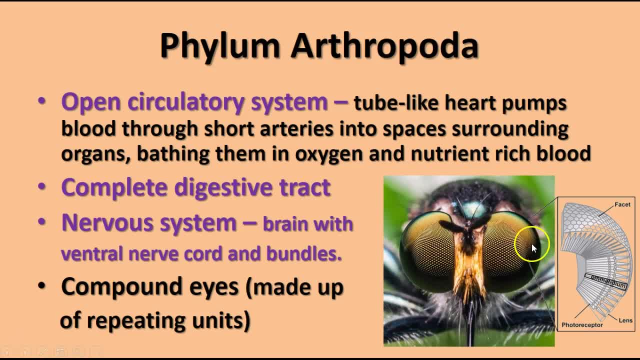 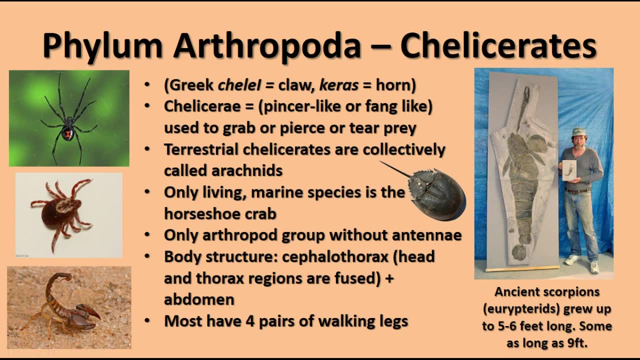 for instance, a fly its greater than 180 degree field of view, because they can see things actually behind them because of the shape of their compound eyes. Within the arthropods we have several different important groups. The chelicerates are animals that have pincer-like or fang-like 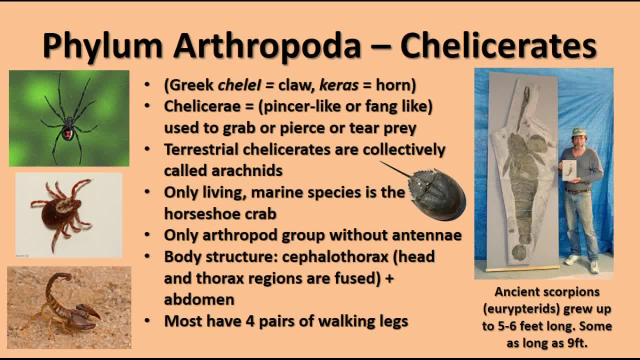 structures that can be used to grab or pierce or tear prey Things like spiders and ticks and scorpions, as well as some less common things like horsey crabs. The terrestrial chelicerates are called arachnids and that includes, as I said before, the spiders, the ticks and the scorpions, The 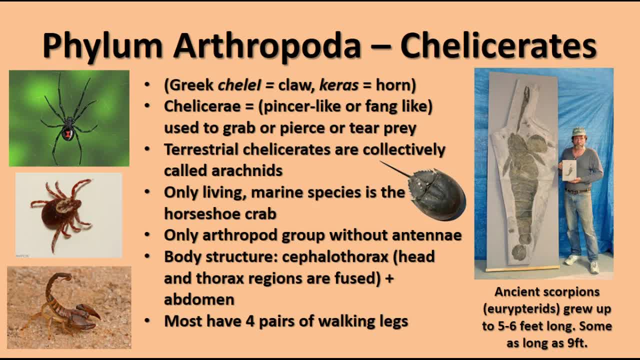 only currently living marine species is the horsey crab, and this is a picture of a horsey crab. Horsy crabs are really interesting. they don't exist in very many places anymore. There are a couple of places along the eastern shore, the Atlantic Shore of the United States, including. 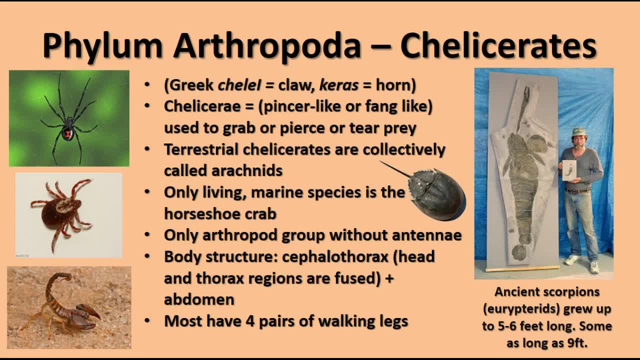 eastern shore of Maryland where you can find horse crabs. The chelicerates are the only arthropod group that do not have any antenna. Their body structure is composed of two parts: the cephalothorax, which is the head, and thorax that are 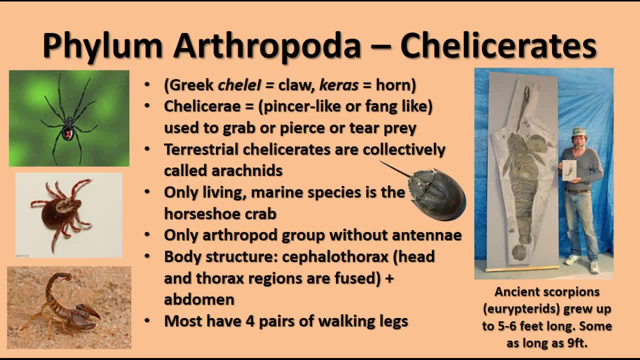 fused together as well as an abdomen, and most of them have four pairs of walking legs. Some of them have several other body parts, like the chelicera on a. on a scorpion, for instance, it looks like the pincers here. This picture over here on the right is a fossil of an ancient 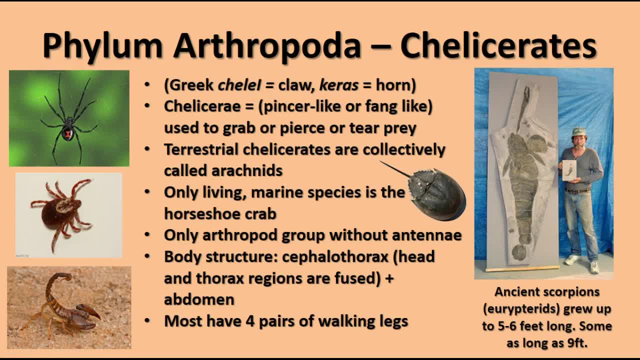 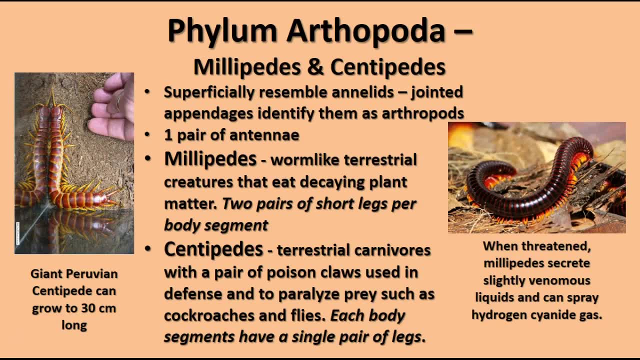 scorpion called a eurypterid that was anywhere from five to nine feet long. Glad they're not around anymore. Phylum, arthropoda and the millipedes and centipedes are the next group If you just look at a centipede or a. 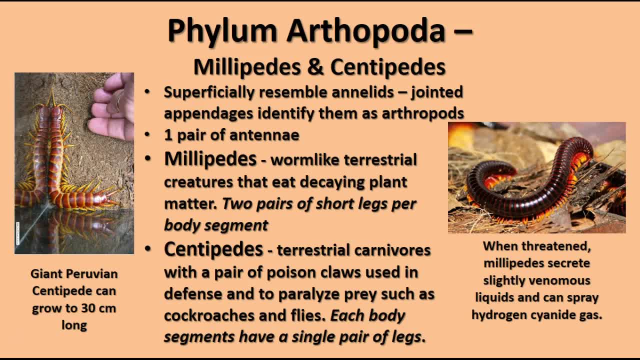 millipede. it kind of looks like an animal. It's actually a genital because it's got jointed body or segmented bodies with multiple segments. but they also have jointed appendages. when you look at their legs, ok, you can tell that they have joints and they can have parts that. 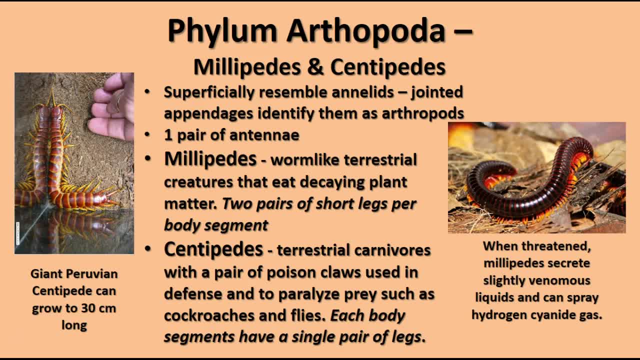 move independently. They have one pair of antenna. The millipedes are terrestrial creatures. they're worm-like, they eat decaying plant material and they have two short pairs of legs per body segment. Millipede means thousand legs or thousand foot, and so they were first born. 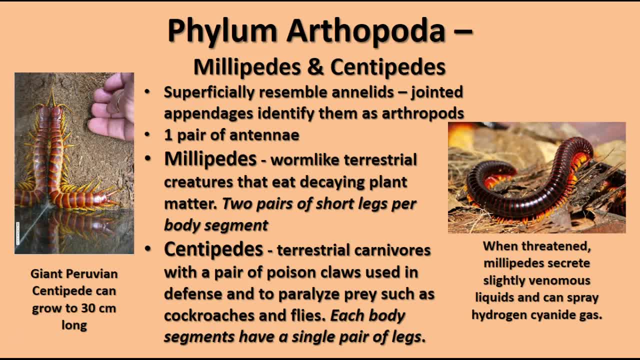 named by people who thought they had, you know, close to a thousand feet. there were so many of them. centipedes are terrestrial carnivores and they have oftentimes a pair of poison claws used in defense and to paralyze prey. each body segment on the centipedes has a single pair of legs. 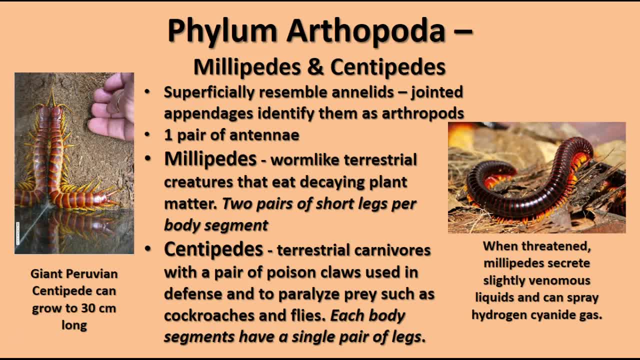 centipedes. centipede means about a hundred foot or a hundred legs, and so they have actually fewer legs than the millipedes do. the giant peruvian centipede can grow up to 30 centimeters long, which is about a foot, and various millipedes can secrete some venomous liquids and even spray. 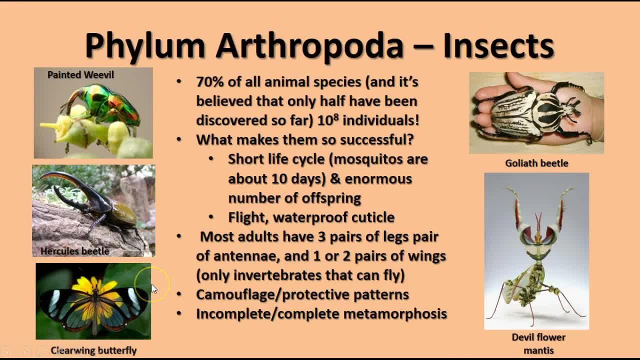 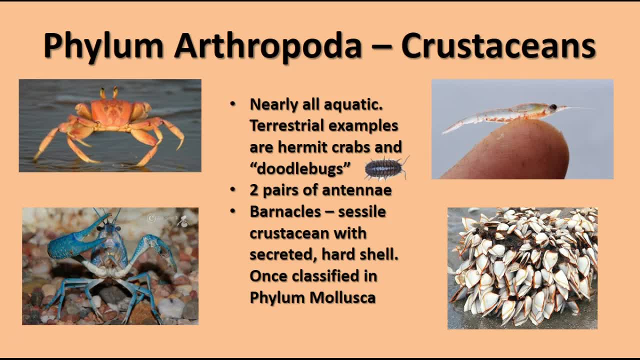 some poisonous gases like hydrogen cyanide. the crustaceans are the next group of arthropods. these- most of these- are aquatic. they include things like hermit, crabs and doodlebugs or arolypolis, as you can see here in the little picture. 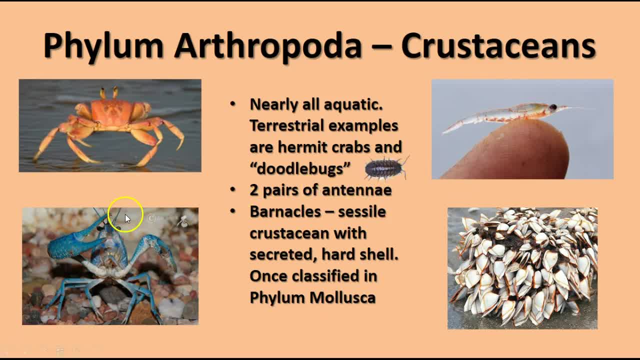 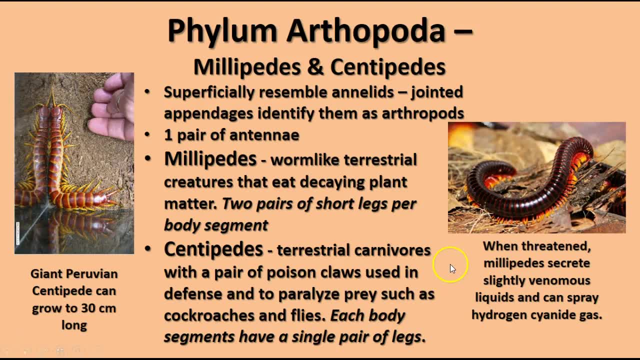 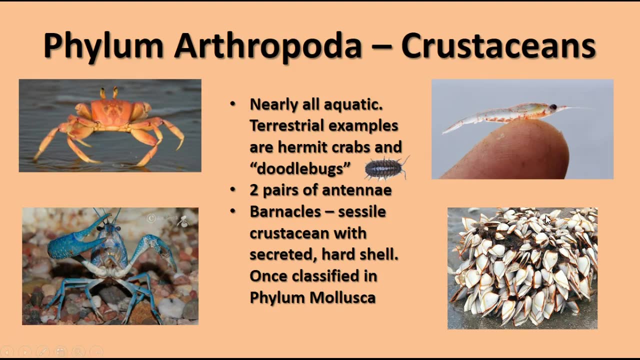 and also things like shrimp, crabs, lobsters and so forth. they have two pairs of antenna and another group that's within this group is called the. it's called the barnacles. barnacles are actually a sessile crustacean, meaning they are rooted to one place. basically they have a hard shell, that is. 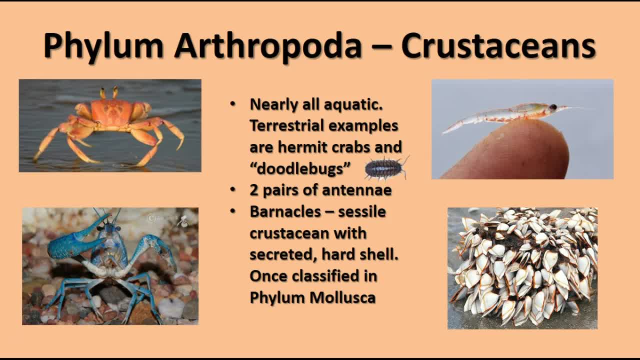 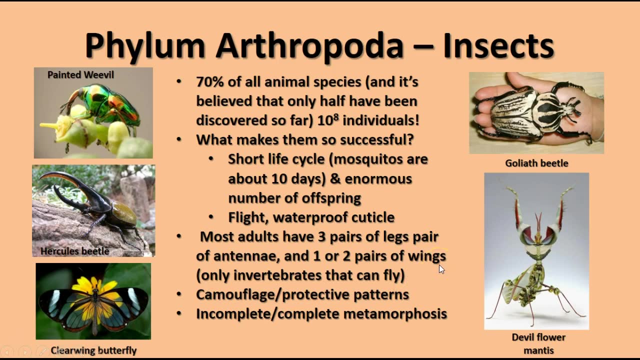 secreted on the outside. they used to be classified with phylum mollusca because people thought they were mollusks, because they kind of look like mollusks when you just look at the shell. but when you look inside the shell you can see that there's a tiny little crustacean in there. the next group with the largest group by far of not. 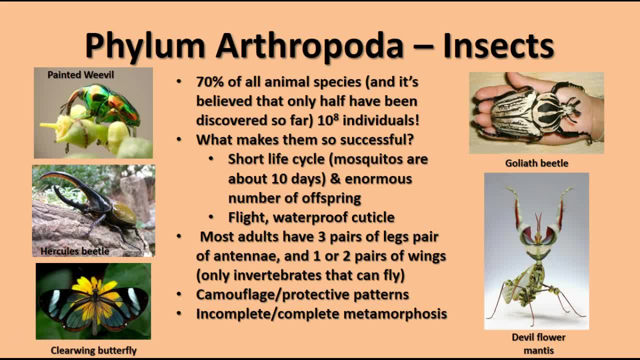 only of the arthropods, but of all animals, is the insects. about 70% of all animal species are insects and many scientists think that we've only identified or discovered about half of the available arthropod species, about a hundred million individual insects. so very, very many of them worldwide. what makes them so successful? well, they have a relatively 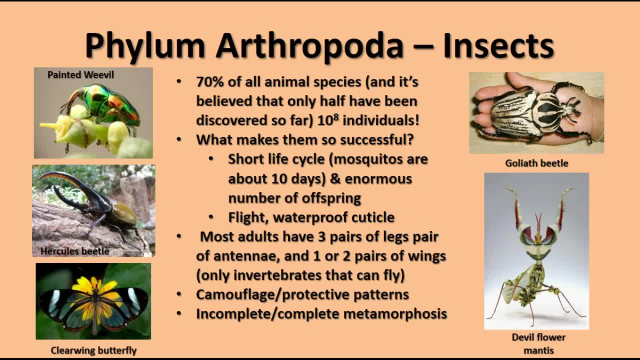 short life cycle. the mosquitoes have a life cycle of about 10 days, and they produce an enormous number of offspring, and so they can. they can reproduce over and over again. they're the only animals- only invertebrate animals- that are capable of flight. not all of them can fly, but 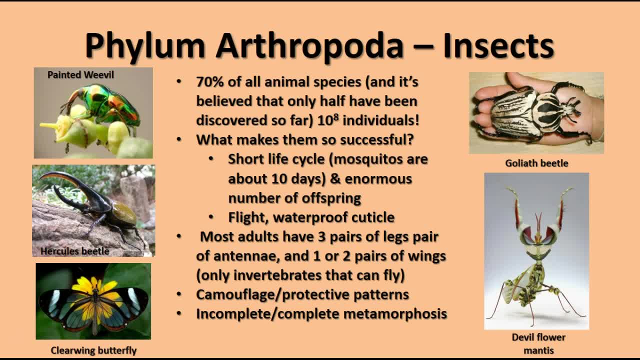 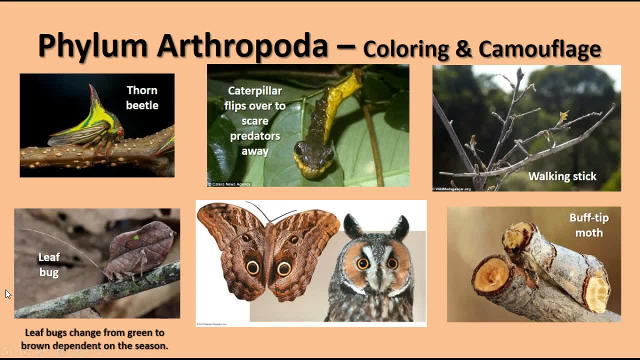 very many of them can. they have various kinds of camouflage and protective patterns and they exhibit either complete or incomplete metamorphosis. here's some of the examples of coloring a camouflage that you can see in various arthropods. here's a thorn beetle, if you can see. if you saw a branch with a. 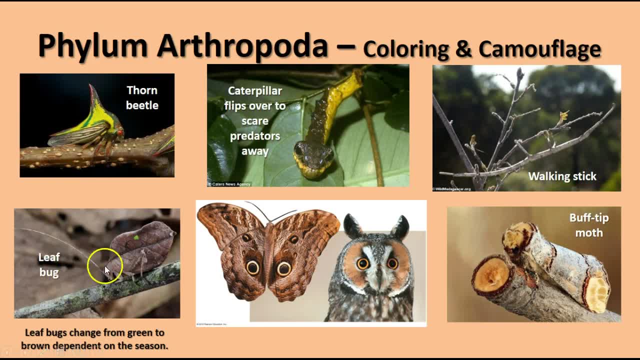 bunch of these on it, you would think it had thorns like a rose. here's a leaf bug, this camouflage like a leaf. they change from green to brown depending on the season. so if it's, if it's springtime, like it is now, they would generally be red. I mean it's green, and in the fall, when they start turning, 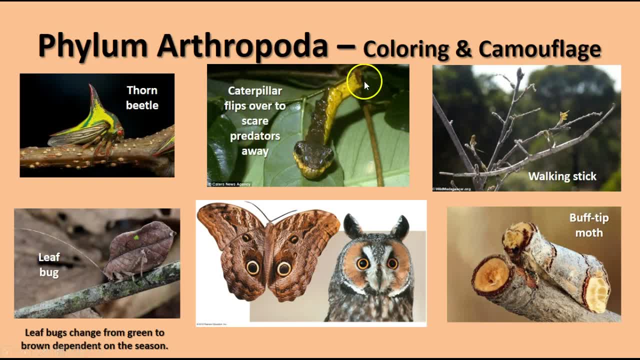 brown, then the bugs will turn brown as well. the caterpillar, this caterpillar here. this is the underside of the caterpillar that looks like a snake, so that would scare a lot of predators away. here's a big moth that has eyes, eye spots that look very much like the owl's eyes, and so predators that might be also. 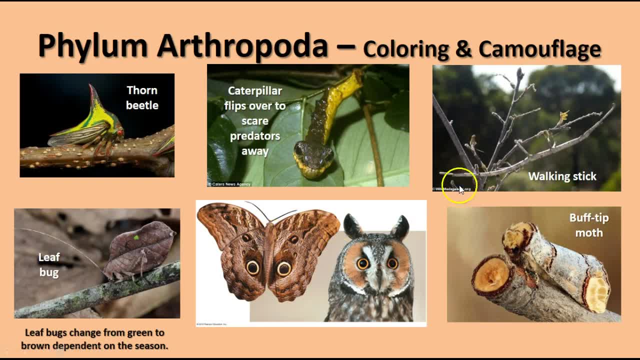 the prey of an owl would stay away from those. here's a walking stick, if you can see. here's the stick insect. it's hanging on the bottom. there's its legs hanging out to this, onto the branch, and here's a buff tiff moth. here's the head of the moth and here's the wings and it looks very.